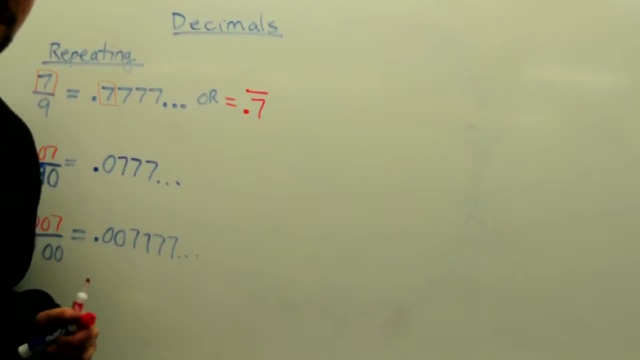 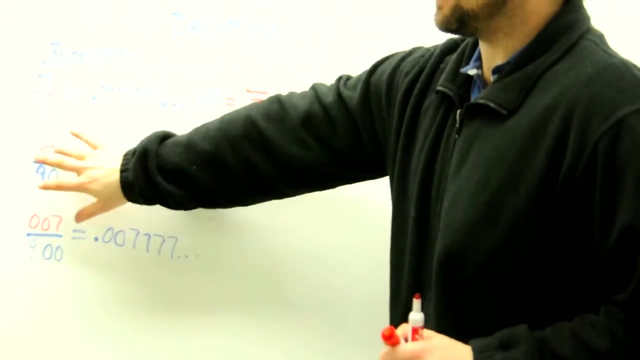 Hey everybody, this is part 2 of the decimal pattern sort of thing. I guess I can move over. So last video we had 7 over 9,, 7 over 99, and 7 over 999, and we had this pattern where we had the 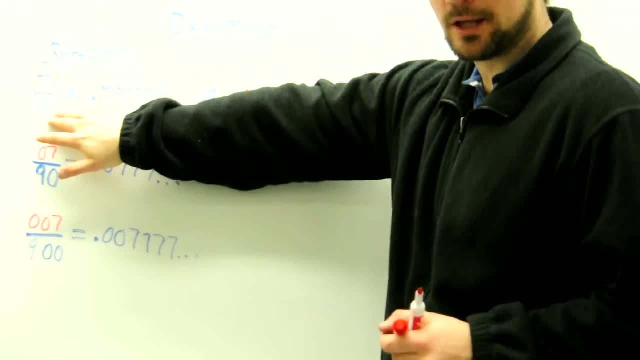 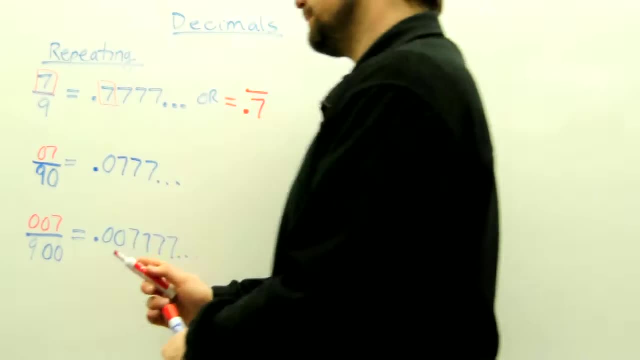 You can look at the last video and check it out This one: here we're going to start at our same anchor point, but instead of 99 and 999, we're going to talk about 90 and 900.. The only difference here is well, nothing really. 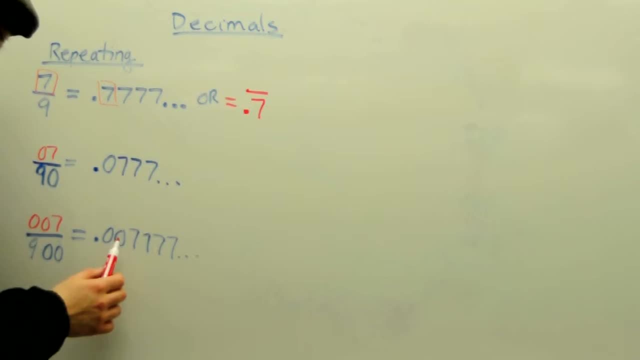 If you were to do long division, this is what you would get. If you were to do long division, this is what you would get, But there's a shortcut, right, We want to look at shortcuts to save time. From looking at this, what are we thinking? 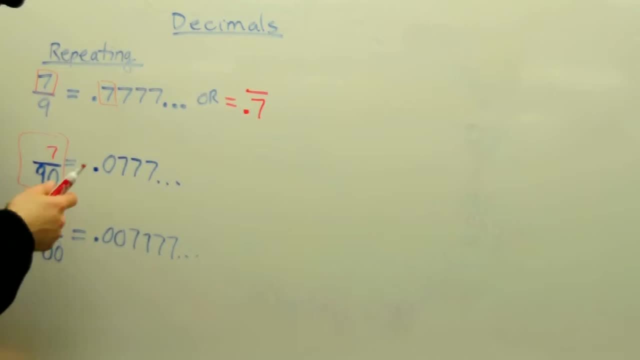 Okay, 7 and 9, so I know it's going to be .777, it's going to be in there somewhere, But this 9 here it's like we're dividing it into one-tenth of the amount. So think of it this way: You put one place, value, expansion- here. 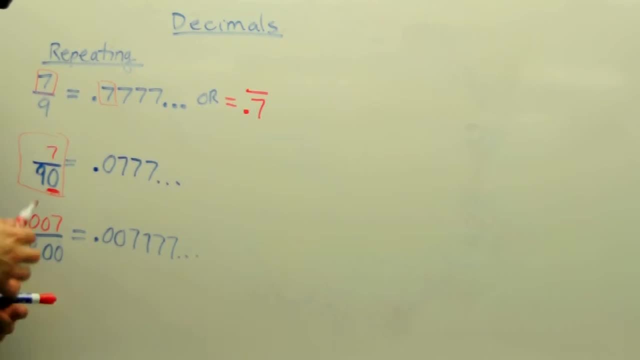 You're dividing it into, you're increasing the amount of parts by 10. Your answer is going to be one-tenth the amount. so that amounts to having your entire answer part shoved over by one place value. So we have a 0 here that accounts for one 0, right there. 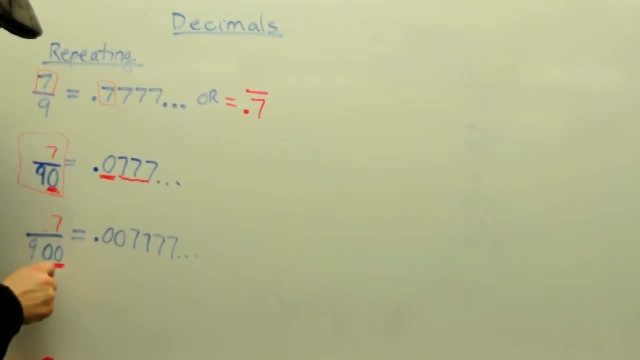 Similarly, here we have two 0s, here, we have two 0s here, And then we get back to the well, 7 over 9 is 7777.. So that's the pattern that we develop here: 7 over 9, 7777.. 7 over 90, .0777.. 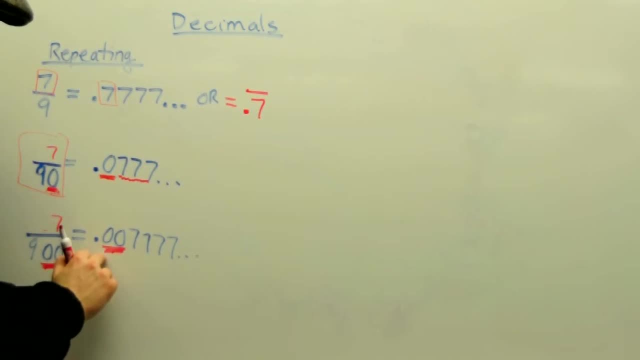 7 over 900 is this. 7 over 900 is .00. blah, blah, blah, Because there's two 0s here, One 0, two 0s. Okay, that's a pattern that will help you recognize things like this real fast. 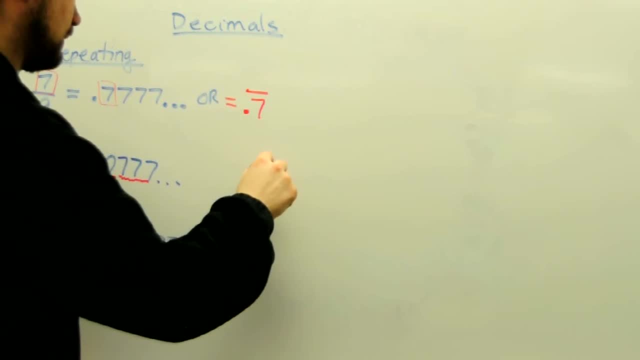 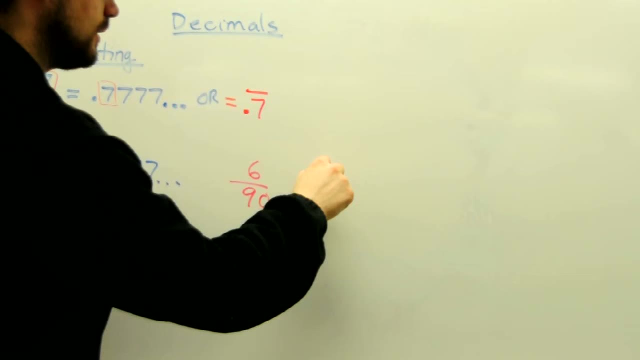 So you could have something like this: Like: how about, like 6 over 6 over 900,? okay, Well, we know that 6 over 9 is going to be .666 and so on. So 6 over 900..